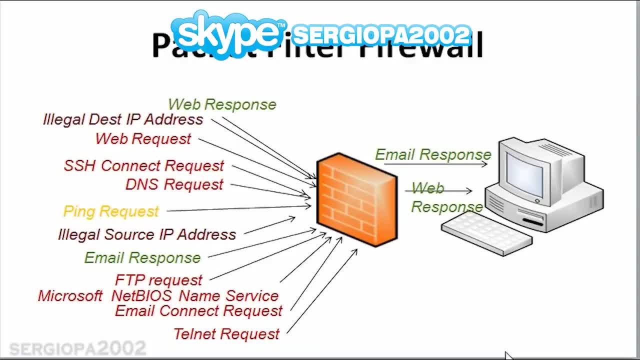 There are different kinds of firewalls. There are purely software firewalls, like the ones we have in Windows 7 or Windows 8, and we also have hardware firewalls, that these are really boxes that have security measures in them. There is also a combination of software and 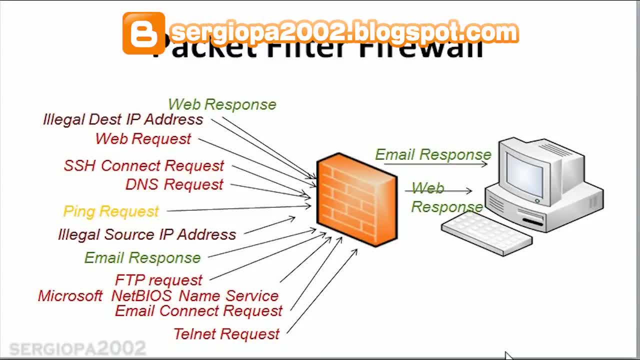 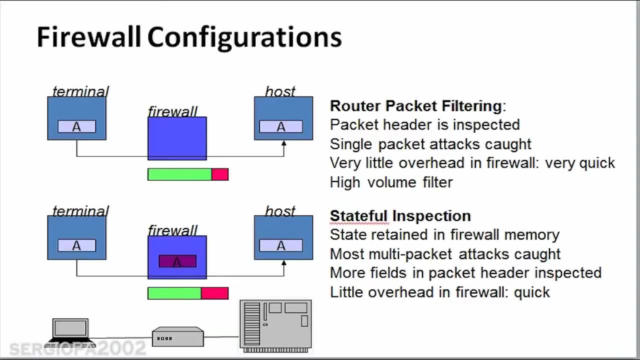 hardware firewalls, and this is normally what is used in networks. Now, that being said, we need to know the different kinds of firewall technologies. So the first type is packet filtering firewalls. In order to explain that, I'm going to show you here that I have in. 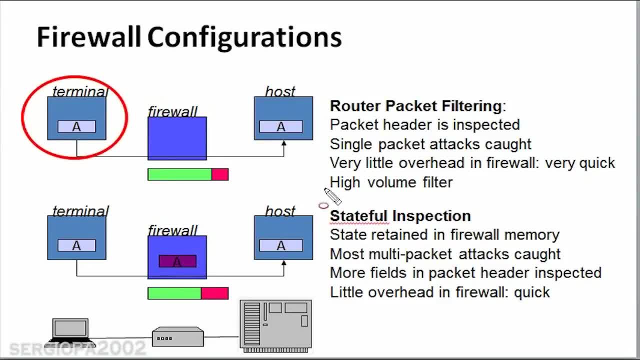 my diagram: a terminal, a terminal computer and a host, And this arrow that you see between them is a terminal, A representation of a message or a package being sent from terminal to host. Now also, you see here this rectangular, here below the firewall, that's our data package, or a zoom. 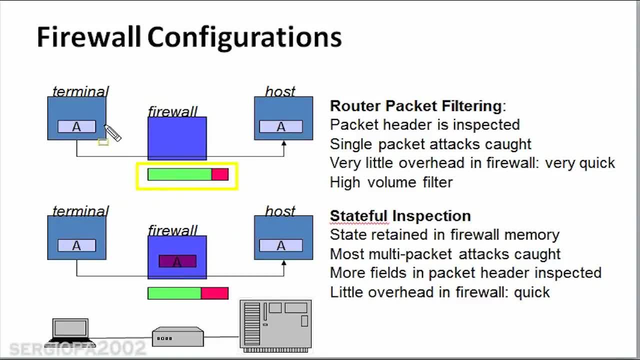 of our data package. Also, you see that this data package has to go through the firewall in order to reach the host. Now, the yellow part that I'm highlighting here, or the red part of the package, is the amount of the data package that this firewall 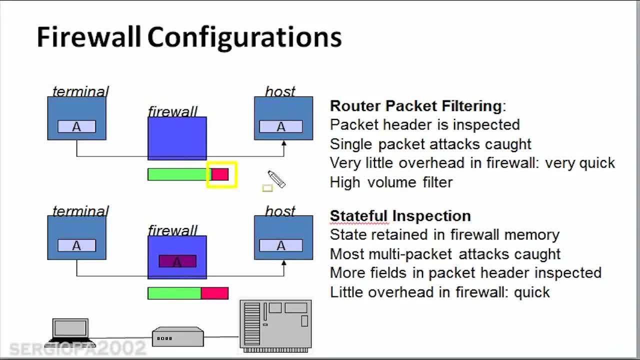 will inspect or check And this will depend on the different firewall types. So in the case of packet filtering firewalls, only part of the packet header is inspected. This means that a lot of packages can go through the packet header. This means that a lot of packages can go through the firewall very quickly, But also means 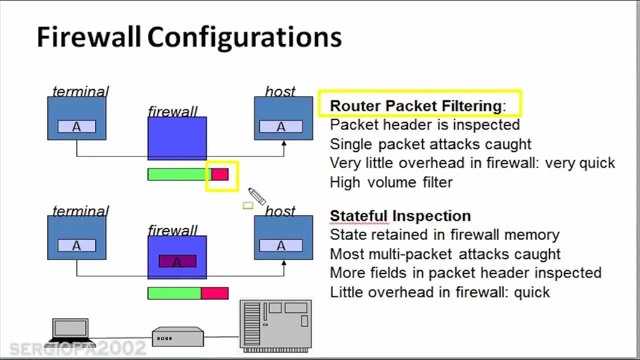 that it's not as secure as other types. It creates very little overhead, so single packet attacks will be caught mostly Okay. the next type is stateful inspection firewalls. As you can see, it's very similar to the packet filtering. It also analyzes the header of the package, but this time it. 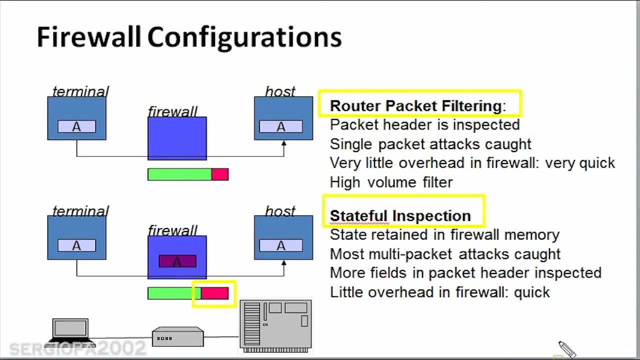 analyzes it more completely. It checks more fields of the data header- Not all of them, but more than just simply packet filtering firewalls. This creates a little bit more overhead in the firewall, making it slightly slower, but it's still very quick Most fields. 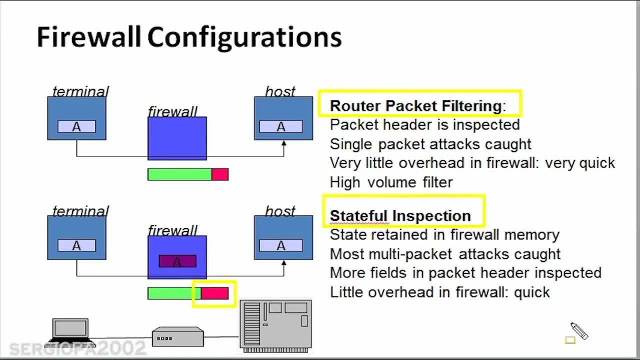 in the header are inspected. but again, it's important to know that not all And most multi-packet attacks are common. This is because stateful inspection firewalls retain the state of the connection between terminal and host in their memory, And this gives the firewall more fields to analyze. 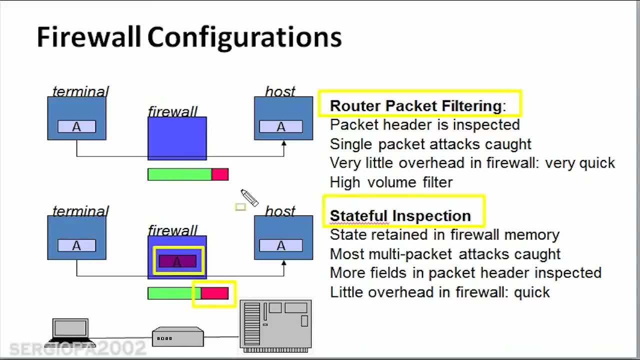 So the states like I'm connected, I'm not connected or this kind of messages that have to happen in communications between computers is retained in that firewall memory and that allows firewall to implement security filters based on those fields or that information, since we have more data to filter. 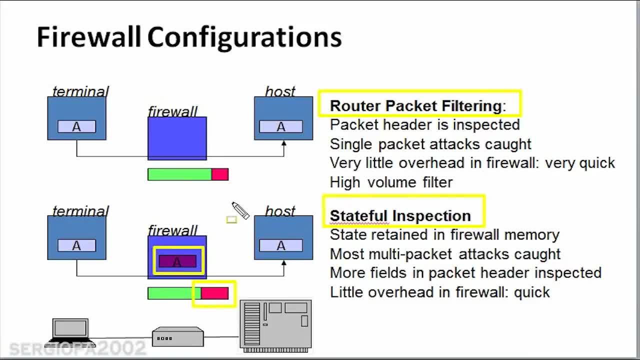 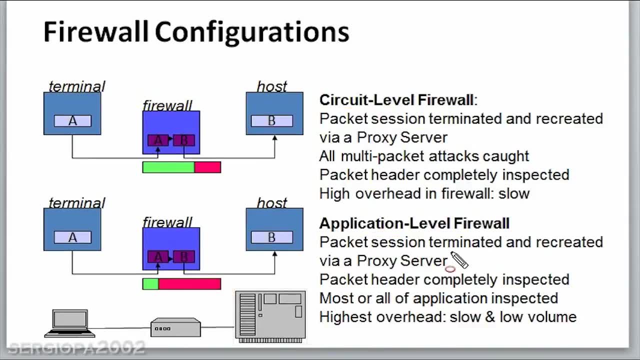 a package is, we are considered more secure than simply packet filtering. the next type of firewalls are circuit level firewalls. in circuit level firewalls you can see that the packet session between terminal and host that needs to be established in order to send the message is terminated in the firewall and recreated. so that's why you see here an a. 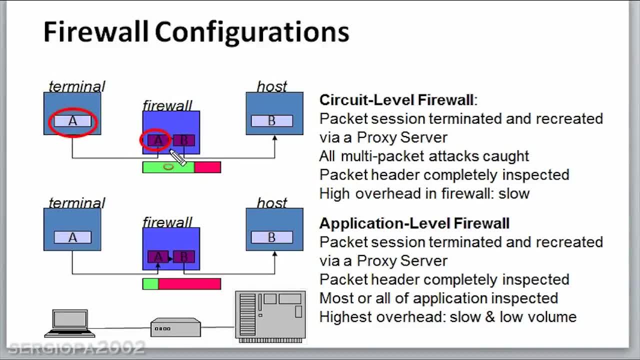 representing the connection and the a here, and then the a ends here and transforms into b, and that b connection is the one that is transmitted. so this adds a additional layer of security to my communication. another important thing is that the entire header of the data package is inspected by circuit level firewalls. 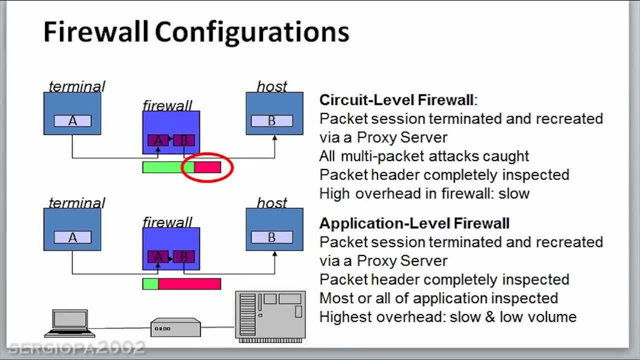 this guarantees that all or most of the multi-packet attacks are going to get caught, but it creates a significant overhead in the firewall, because creating this- terminating this session and recreating or restart another session- it takes a lot of work. of course, this gives an additional level of security.